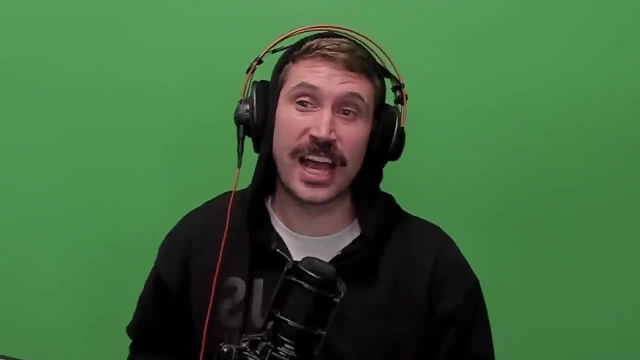 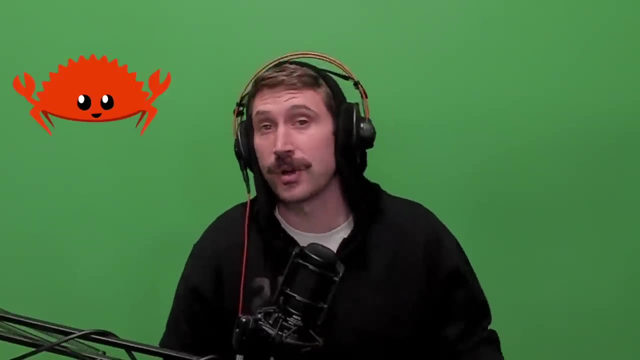 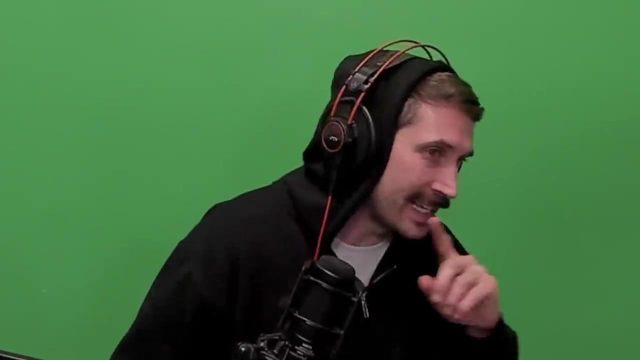 so i have been programming professionally and on the side for getting close to two decades at this point. i've spent many years writing java c, c plus plus, python, rust, go, javascript, typescript, you name it. if i could go back and correct one mentality of mine from that entire time, i know exactly. 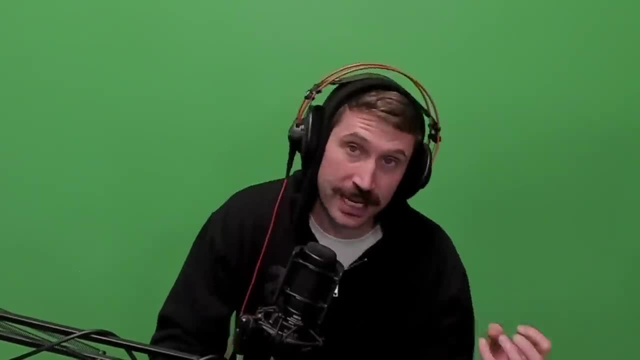 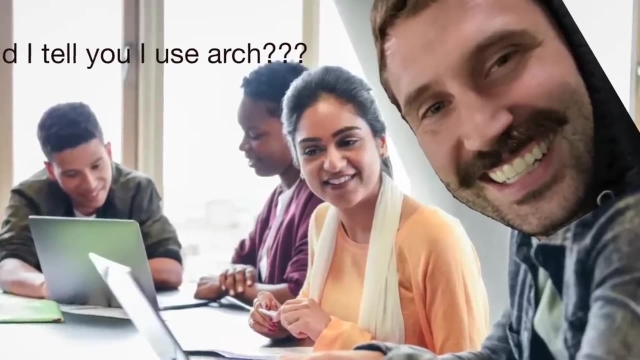 what it would be. so first let me tell you a story so that way you can kind of understand where i'm coming from. in 2007, eight nine, i was in college. i'm pretty excited just learning how to program getting pretty dang fast. you know, i did a little bit in high school. i did a little 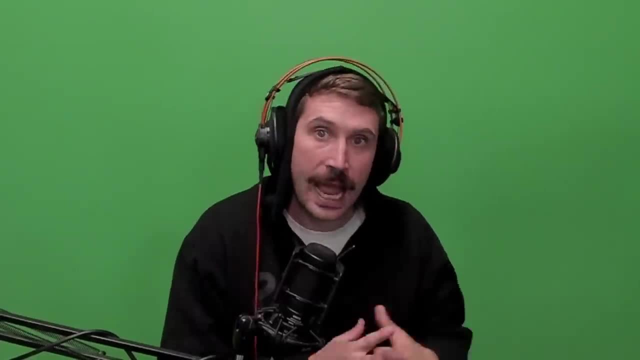 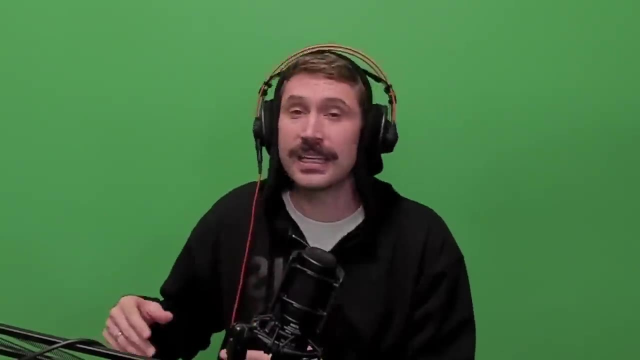 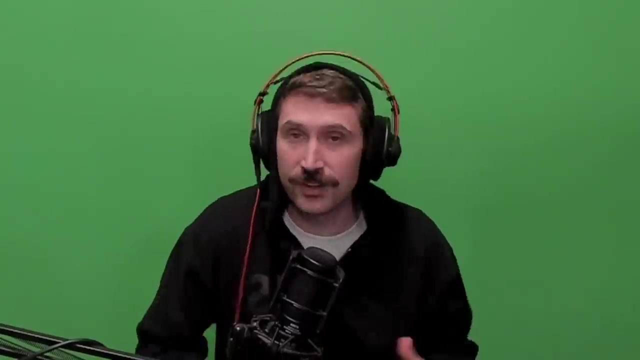 bit of it when i was, like you know, in sixth grade. but now i'm really actually doing it and the thing is is that i've always been on a windows machine. at that point, i just loved, obviously, gaming. that was my thing. oh, oh, you almost got me trapped. oh, i had a lot of fun doing it. 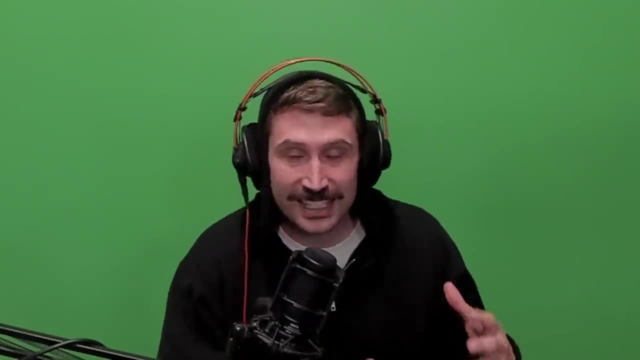 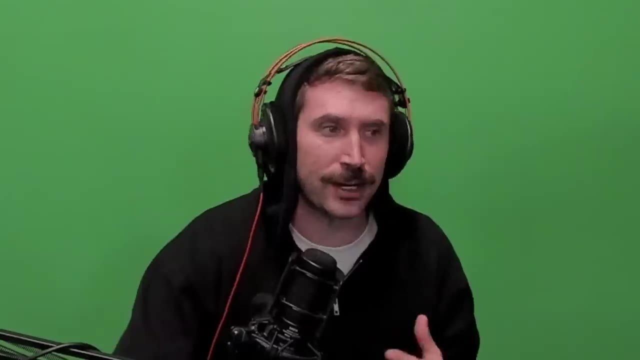 and now, all of a sudden, i'm in college and that's still the operating system that i prefer. of course, a lot of my classes and everything require me to use centos or centos. i can't, i have no idea. the fresh maker, i have no idea how you actually say the thing, but either way i, you know, would. 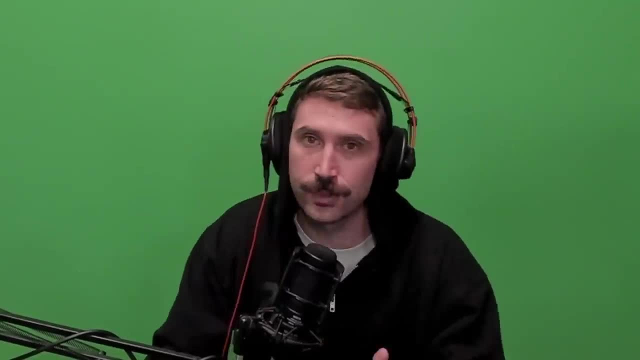 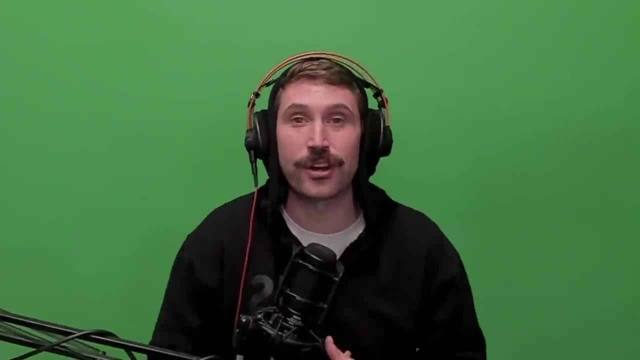 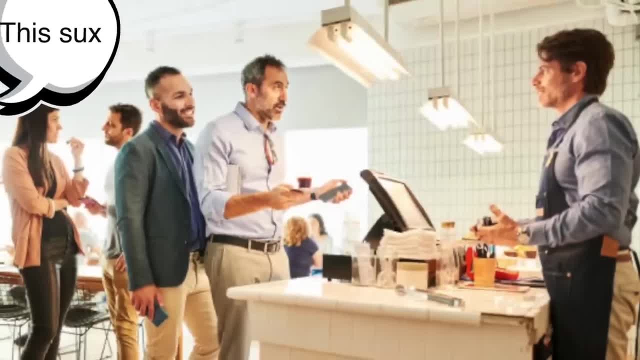 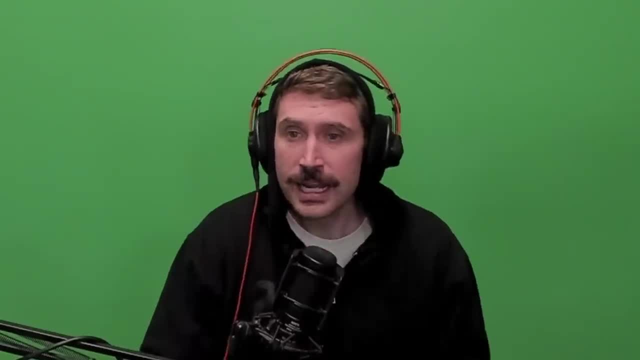 notes about things that are hard in america, such as having to wait in line for coffee, as you know, those kind of things, right. anyways, while i was developing it, i kind of had this idea: okay, i kind of want to get good at linux, and so, in 2008, got partitioned by machine, put ubuntu on it. 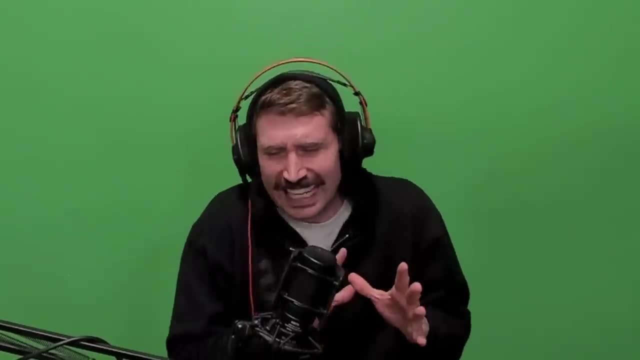 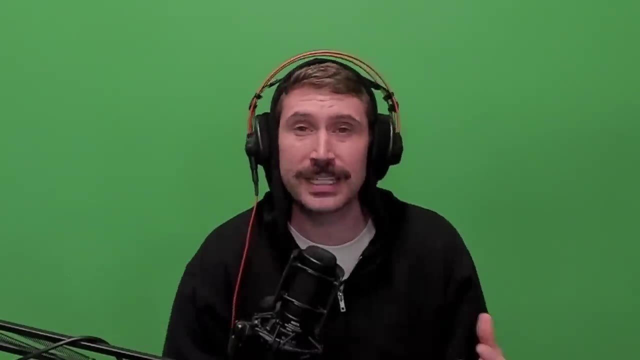 and i stuck with it for probably about a week, but i just i kind of like avoided it- you know what i mean- like, yes, i was using it, but i really just avoided it. i didn't actually do it and ultimately i stopped using it. all together, i kind of had this mentality that i 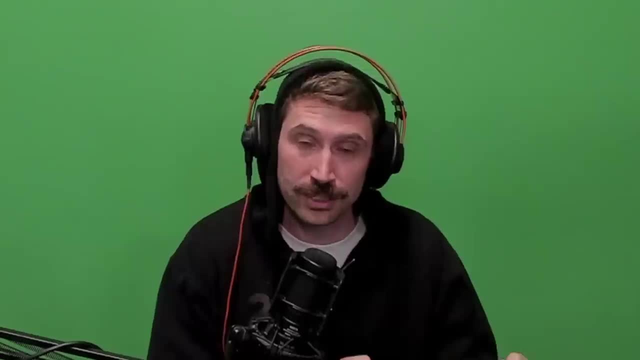 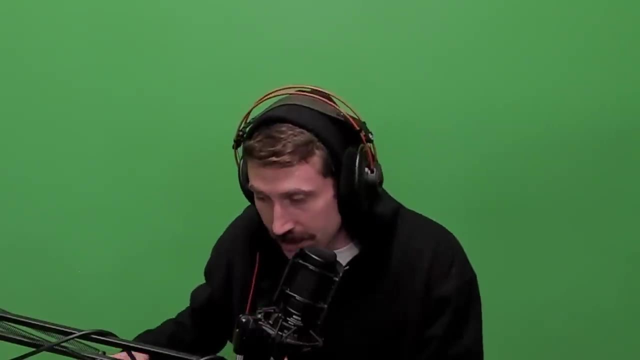 was right and when i looked at things that had some sort of friction or difficulty to them and i could kind of perceive it, i would just assume they are wrong. and what i mean by this, of course, is like using the cli or vim or any of you know, kind of like the more hardcore. 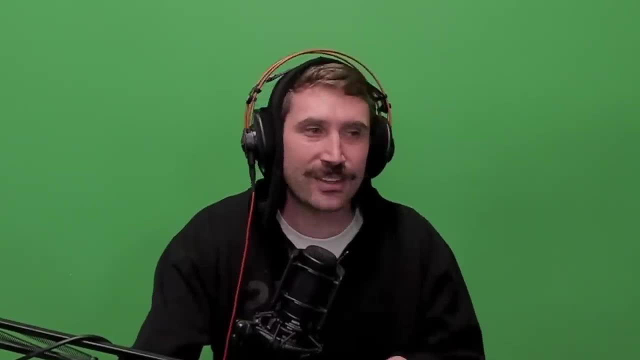 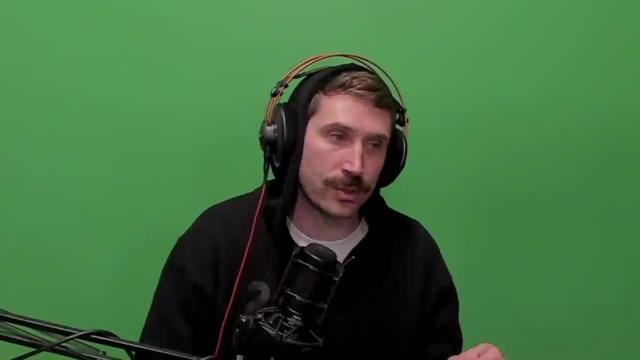 hacker type things. it just felt like they were kind of a thing of the past, a relic of the past and really the futures in these ids and that is it, and i didn't realize how much that was going to hinder me for quite some time, uh, for many, many years. i just simply 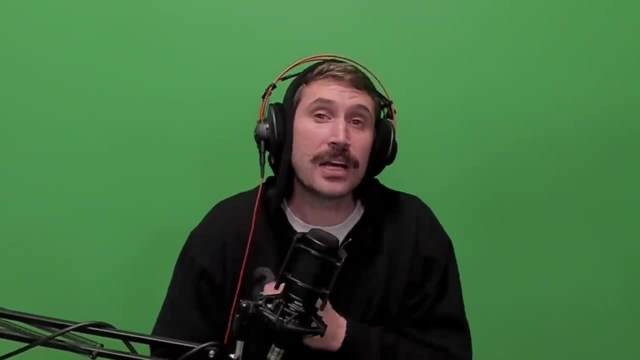 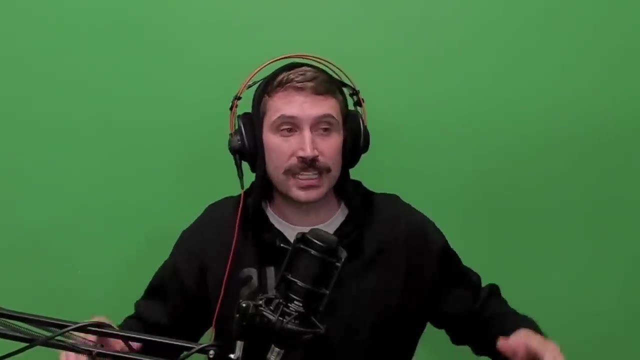 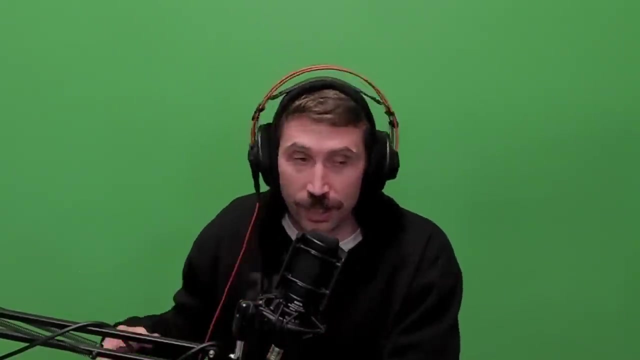 avoided all these hard things, uh, things that were different, not because they were not beneficial, but because i simply assumed they weren't beneficial. i had this mentality where i believed i was right. and that didn't just stop with the technologies i used. it also happened to be when i was at work. 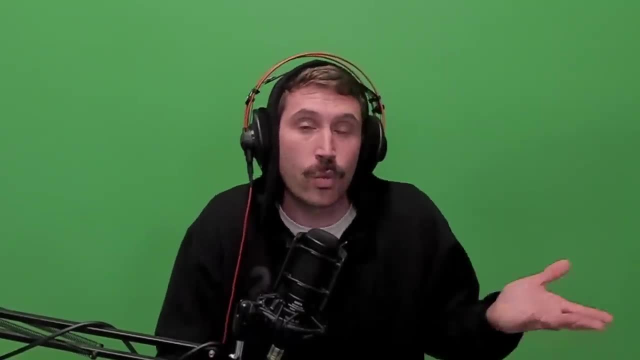 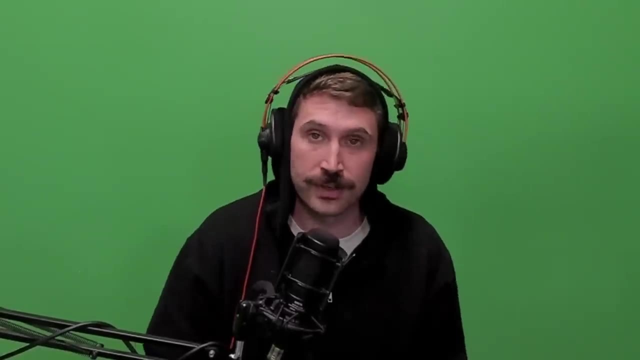 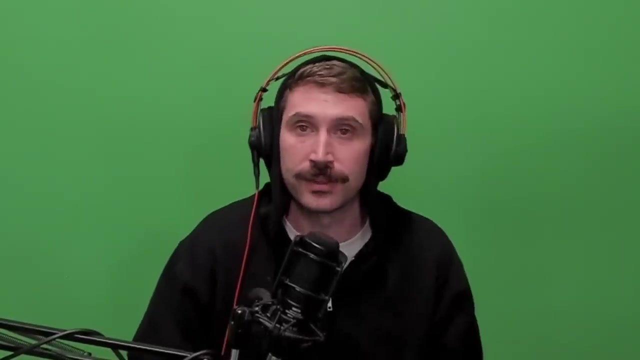 how i treated people, all those kind of things. right, because it all is one mentality. i simply believed myself to be more correct more often than others in all sorts of areas. and yeah, i was pretty smart, i did the best, top of my class. i was obviously very good at my job, excelled above. 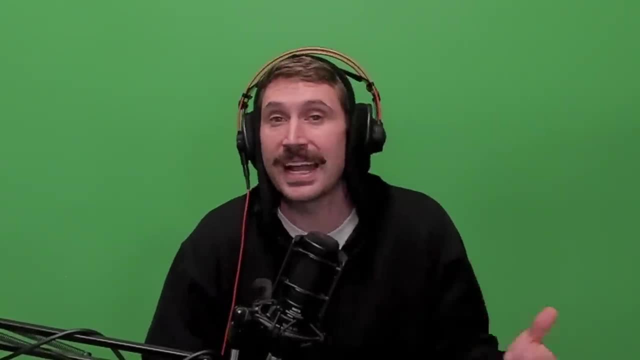 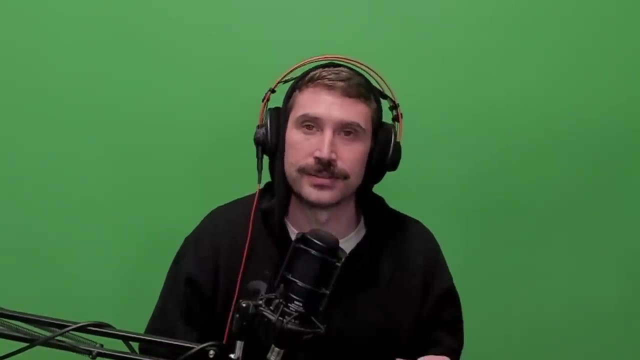 other people, confidence kind of, you know. even though it was a bad type of confidence, it kept compounding in on itself and if i could go back, i really just wish i could tell myself: you know, it is okay to be uncomfortable, it is okay to use something that is perceivably slower than what you 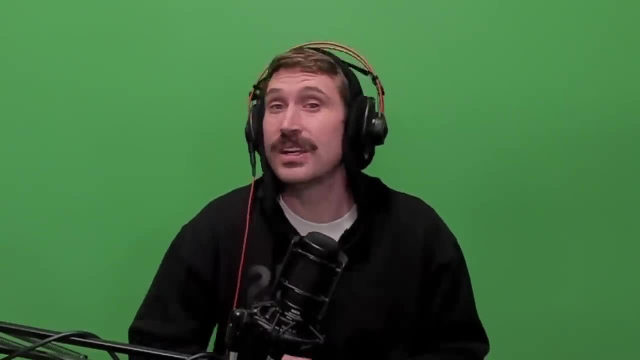 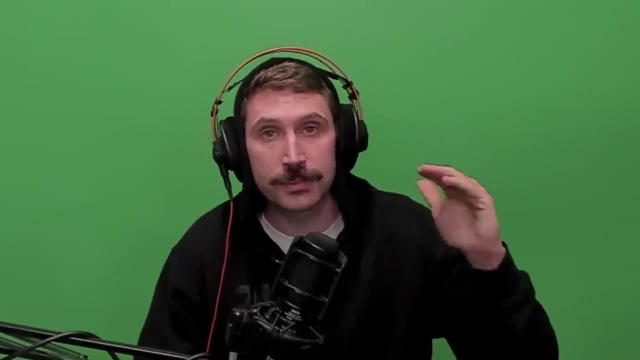 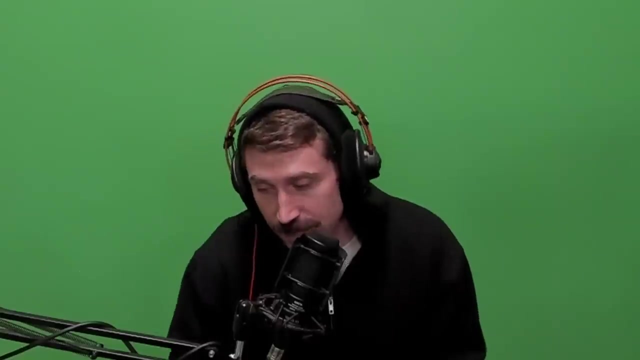 use right now, or even way more difficult, to do the same thing, because it's not about your instantaneous speed up, it's about that long-term dividend play. if i would have known this, i would not have had nearly as bad of an interview as i did for a company i had. they asked me: hey, could you go through a directory? and 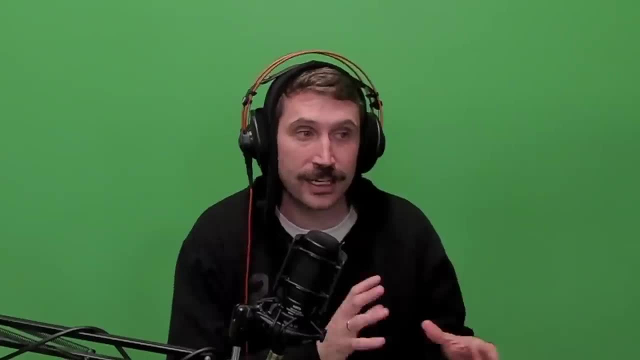 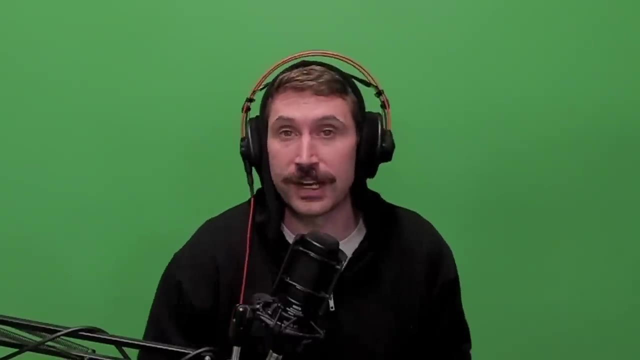 it has sub directories and all these different files have- uh, you know, just have a bunch of html and all this, but we've been hacked and there's a bunch of free viagra- call this number- throughout all these different files and we'd like to remove all of them now, of course, me being the young. 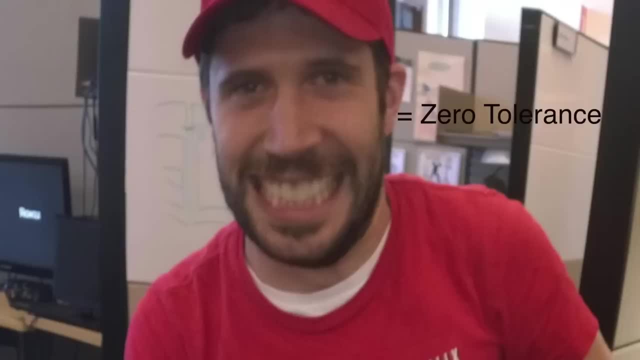 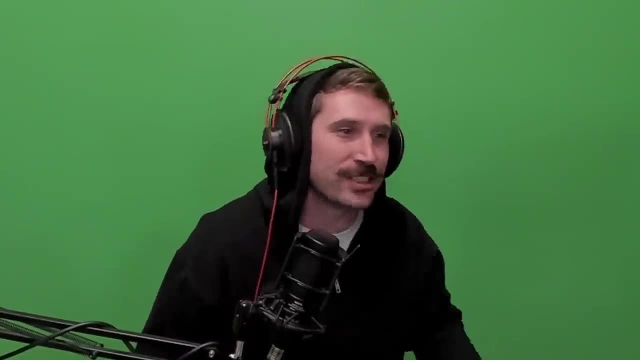 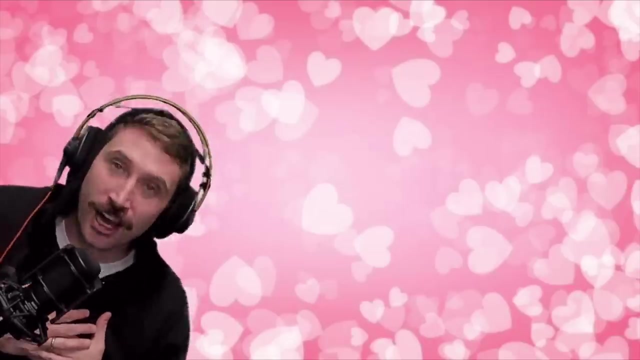 spitting engineer with zero tolerance for the cli and those other things. what did i do? i, literally by hand, wrote perfectly working java code buffered writer tokenizer. bam bam, bam, bam, bam bam wrote the entire recursive directory: walk from my heart of hearts onto the board. and, of course, what did my interviewer do? 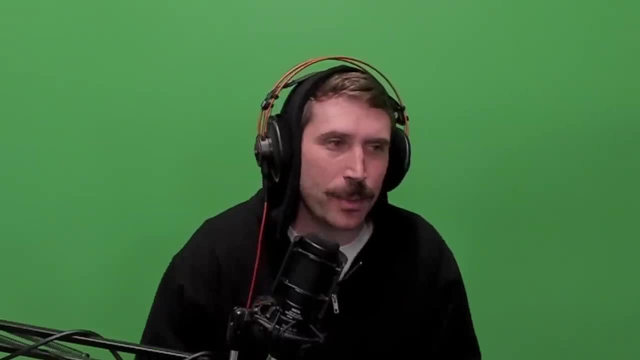 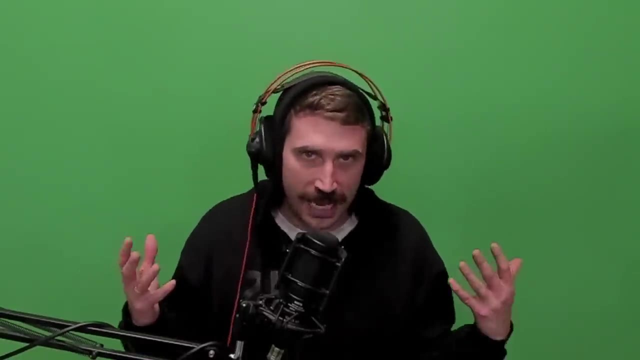 you could have just used grep, and it was kind of like in that moment i realized i should probably know more. right, because looking back on it it's obvious i know exactly how i would solve that. now i'll you know, boom little said grep, super combo, right, it'd be super easy to kind of go through. 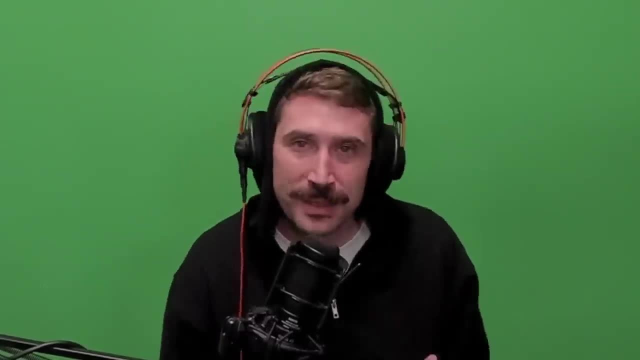 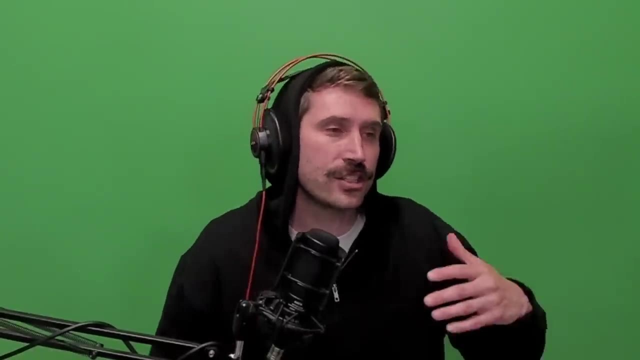 some stuff and just depending on like if you just want the list of files or do you want me to change them right, and so i kind of feel stupid right now looking back, and so i really hope you can hear this. it's not just me trying to get you to use vim or saying the cli is the best place, but really. 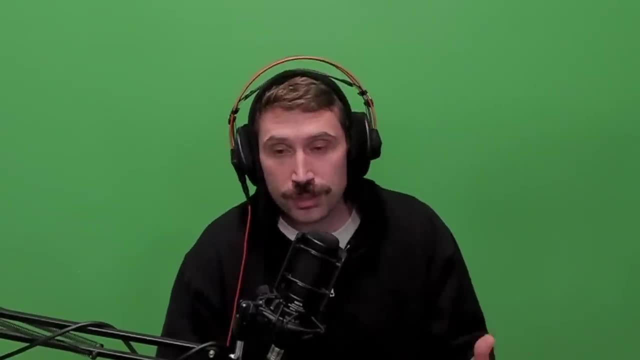 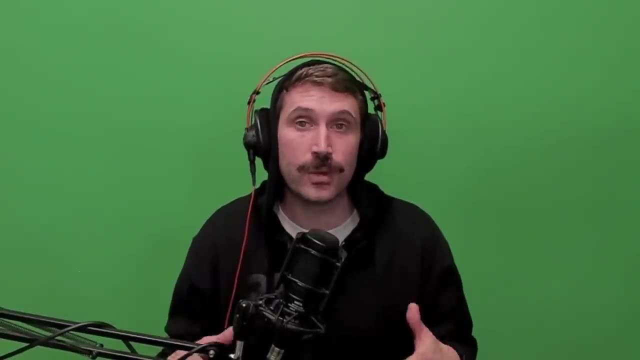 for you to look at problems and understand that you don't know everything and that using things that seem different or strange it's okay because ultimately it's going to be the best place for you, gonna make you a better engineer and, who knows, it may pay some amazing dividends down the road. and 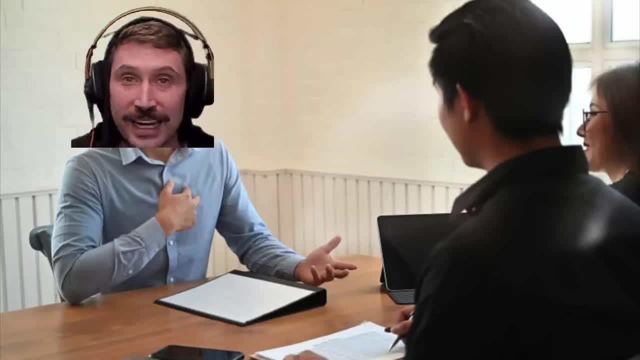 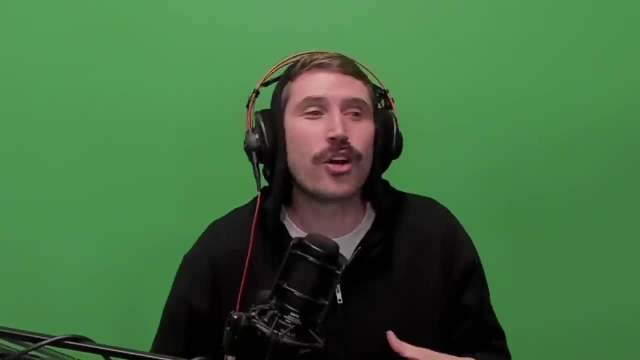 hopefully you don't look like such a doofus as i did during that interview, so go ahead. if all you ever use is vs code, try emacs. look at this. i'm not even suggesting my favorite editor, vim, at this point. go just try anything else. go try intellij, go try some other things. see what you can do. 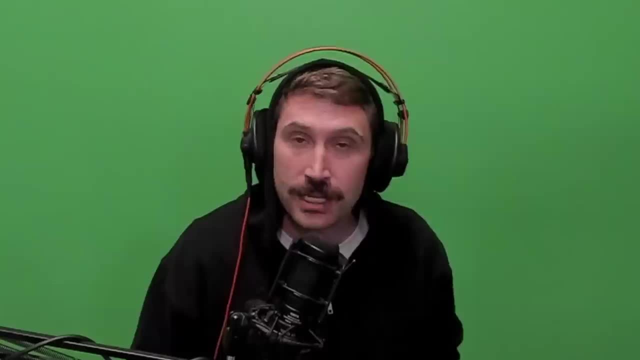 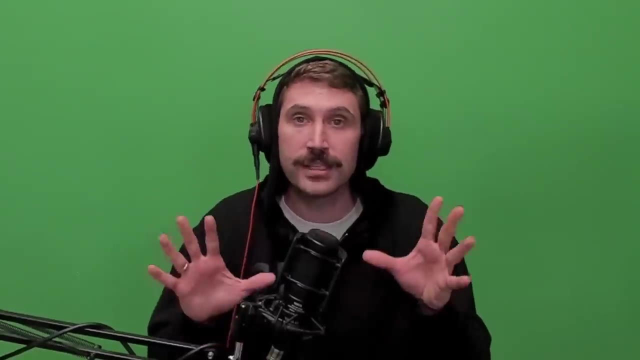 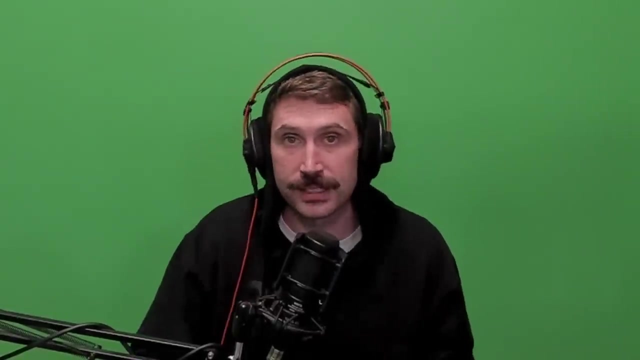 your. all you ever do is just do react and front end, try solid, try view, expand your horizon, try to understand things better, because, ultimately, the more ways you see a problem be solved, the more ways that you can solve a problem. we are often limited by our experiences, and that's really what separates a junior from a senior, is just. 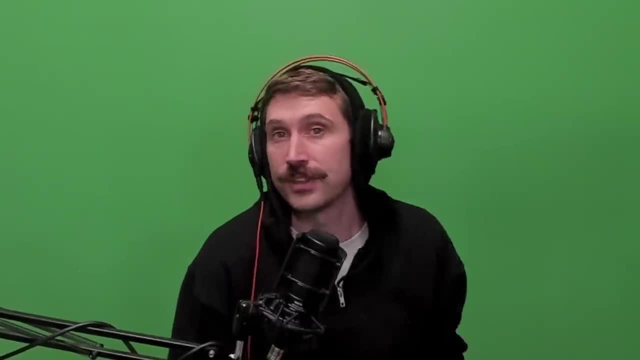 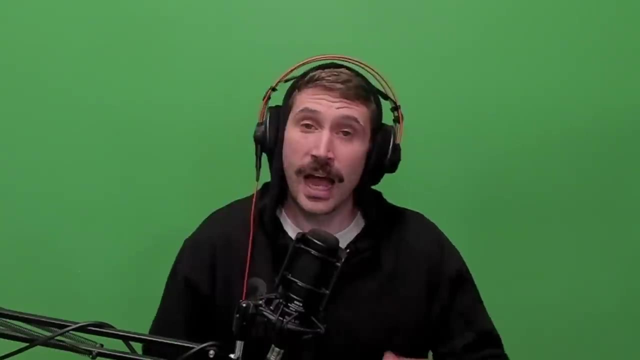 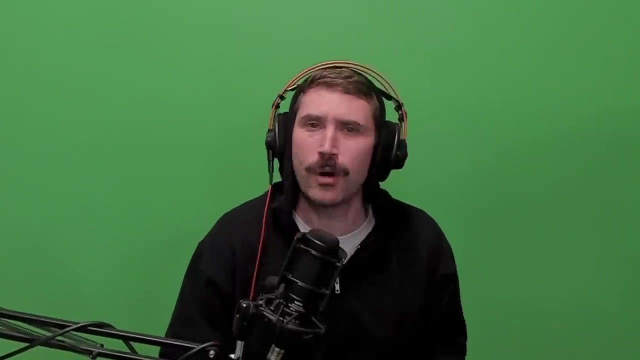 experiences, experiences seeing things done differently and ultimately, that's going to make you a much better engineer, and i really wish i could have told myself that a decade ago. i hope you liked this video. please subscribe and, of course, actually make a comment down below. tell me a little story about yourself. i probably will. reply to you. my name is the primogen.